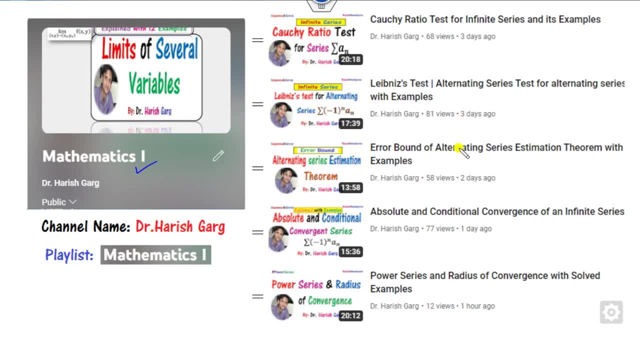 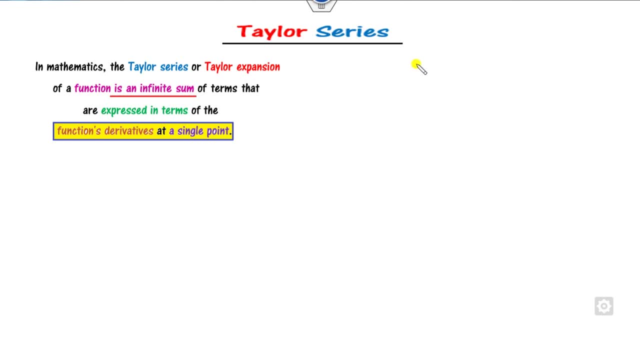 find this playlist mathematics one under the channel name Dr Harish Gaur, where you can find the previous lecture. Now, in this lecture, we will see what is the Taylor series and how you can find this for the function, any of the function. What is the Taylor series? It is a function. It is an. 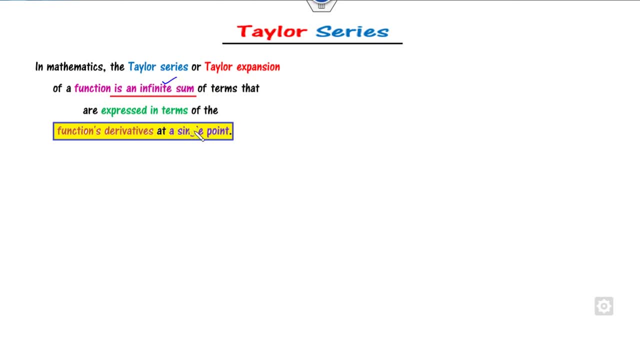 infinite sum of the function which can express in such a way that a function f of x has infinite derivatives at a single point. If I say the point is my a, then you can find the f dash, You can find the f double dash, triple dash, and so on up to the nth derivative at this point, This Taylor series. 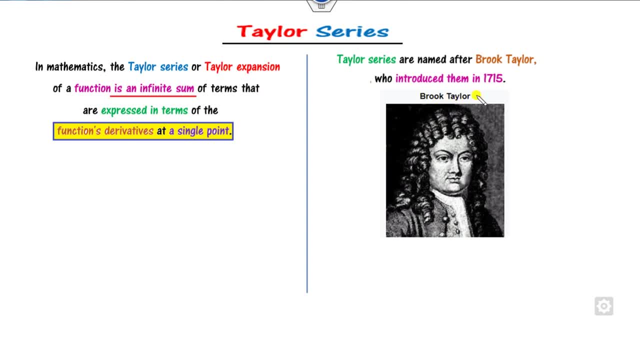 is introduced by this person called as the Brooker Taylor in 1917 under 15.. If you consider the single point as a origin, or you can say, if I say single point is x is equal to a, if I reduce them to the x is equal to 0, then we will call as the 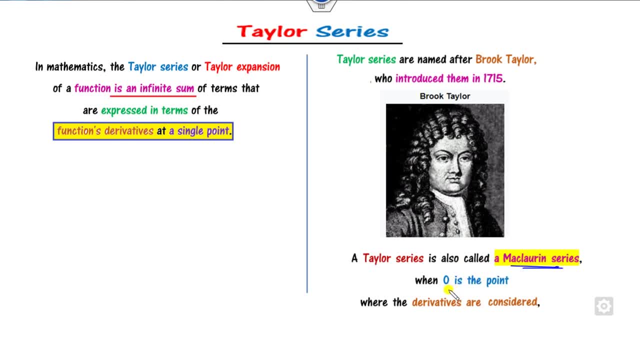 Maclaurin series. That is it. in this case it is a. 0 is the only point where derivative considered For most of the functions. whenever you are talking about the Taylor series, the function and whatever the sum are nearly equal. We will discuss this concept in the couple of this presentation. So suppose you have a function f and 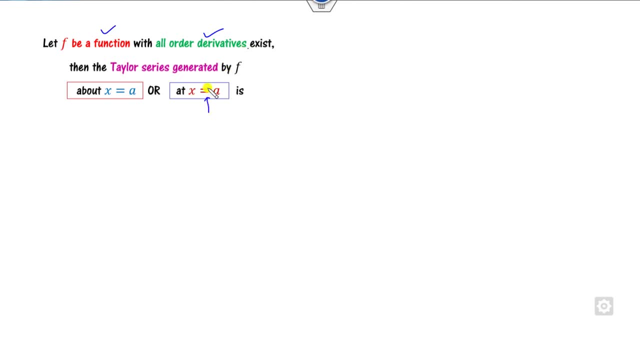 whose all the order derivative exists at the point a or about the point a. then you can define the Taylor series. For example, if I say this is my ln of 1 plus x, clearly say that this is not defined when x is minus 1.. It means Taylor series is not applicable at x is equal to minus 1.. However, for 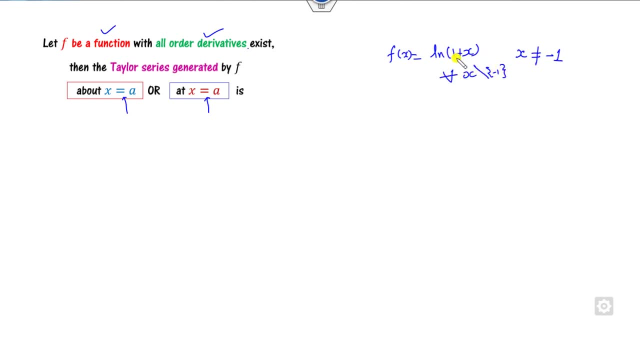 all those x apart from this minus 1. this function is well defined, so you can define the Taylor series at this domain. What is the Taylor series is, if you define the function f about the point x is equal to a, then we can define like of this f of a first derivative over 1 factorial x minus a second. 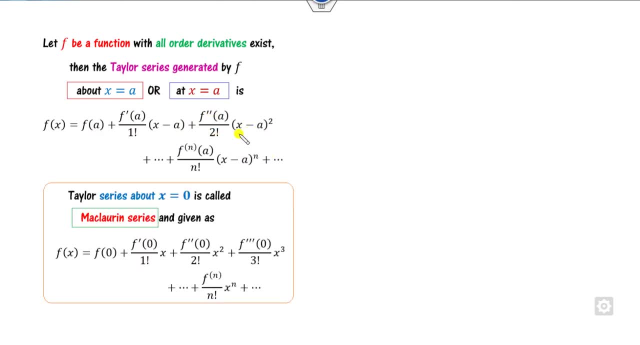 derivative over second factorial and so on. this case, If I consider the point this is my 0- then we call as the Maclaurin series. The basic advantages of this Taylor series is based on this Taylor series we can express any polynomial f of x as a power series. that is a major advantages of this Taylor series. So you can take any of the 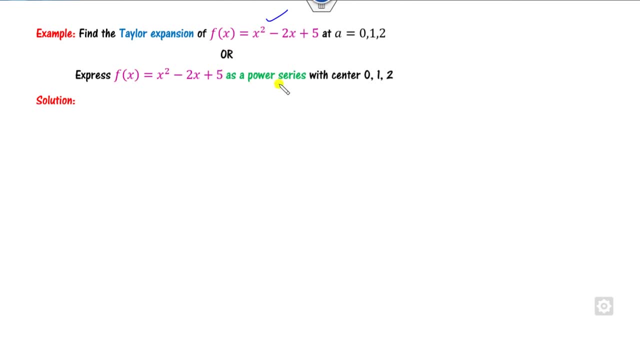 polynomial f of x, like here, you can express in terms of the power series, with the center 0, 1, 2.. How you can do that? that is a very simple: your target. this is my power series. So what is my objective is your target is to change if I say I want to. 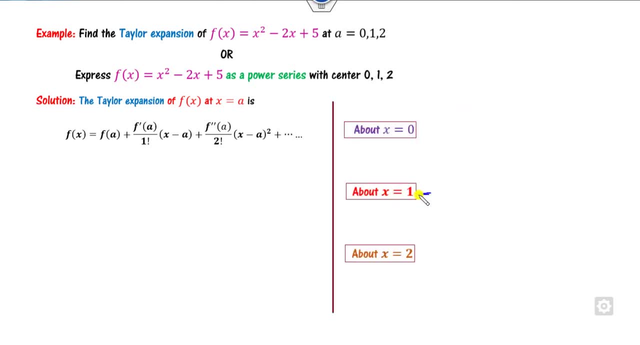 be the here say about the x is equal to 1. what is the meaning? I can change this one in such a way that everywhere, x to be changed as a x minus 1, plus constant. So these are these. what is the coefficient of this? similarly, about x is equal to. your target is to find these coefficients. 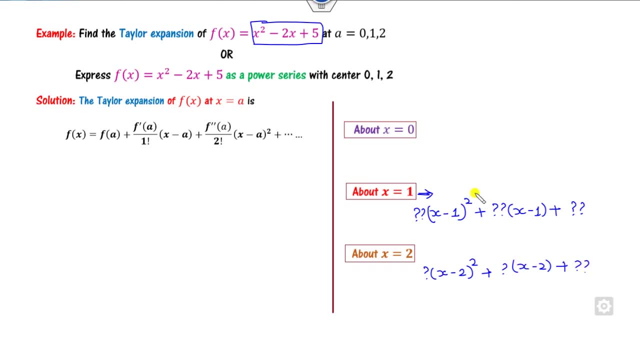 How you can find that this is the target and this will help by the Taylor series. So now, what is the meaning of the x equal to 0. So if you substitute here, firstly you can find the derivative of this function, and here, after that, all are my 0 about x equal to 0, you can substitute x equal to 0 here. 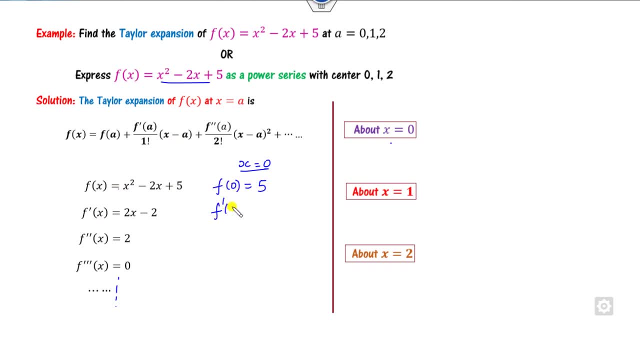 So what is the value of the f 0, that is 5. what is the value of the f dash 0 is a minus 2, and so you can substitute the value here you will get. this is f of 0, that is a 5. this is minus of 2, that is 5. 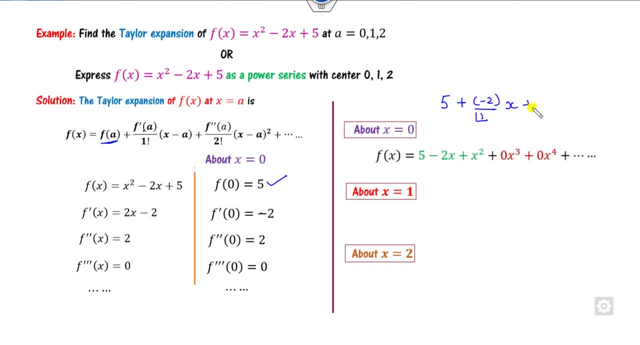 minus 2 over 1. factorial x plus 2 over 2. factorial x square plus 00, and so on. So 2 upon 2, factorial is my 1, and so on. What is the x equal to 1? it means you have to find this derivative at x equal to 1. these are my here. 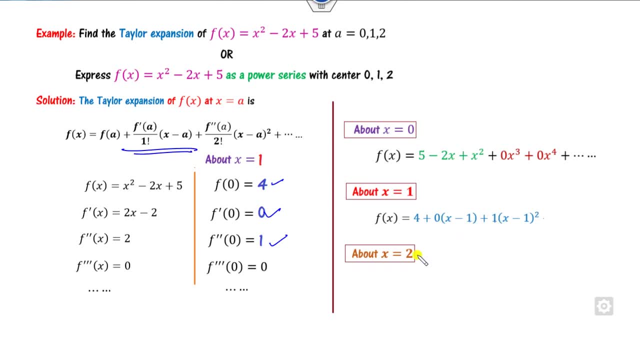 substitute this value, you will get these coefficients. Similarly, about x equal to 2, you can find these coefficients here. you can substitute here, you will get these as the required functions. So this is the way you can. sorry, this is my 1.. So this is the way. 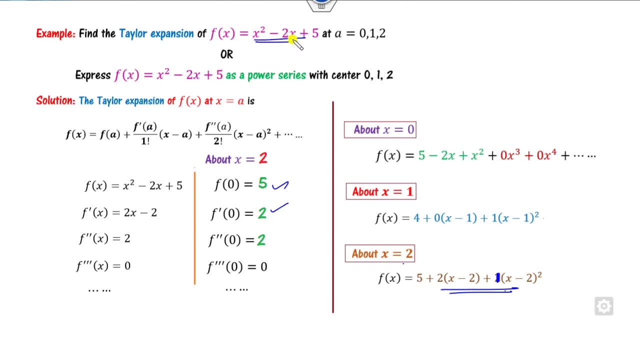 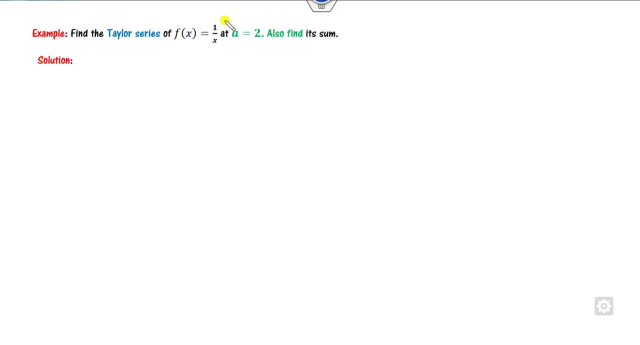 can find, express any of the polynomial with the help into the power series, with the help of Taylor expansion. Apart from this, if you have some another known polynomials like 1 over x, sine x and so on, you can easily express in terms of the power series. For example, this is the 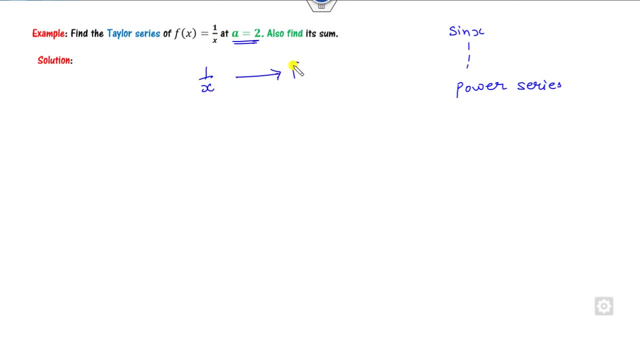 function 1 by x. your target is to make them as a power series. you can make them as a power series with the center is my 2.. It means your target is to express this: say some constant as f of 2 plus the constant x minus 2, plus constant x minus 2 square, plus constant x minus 2 raised to power. 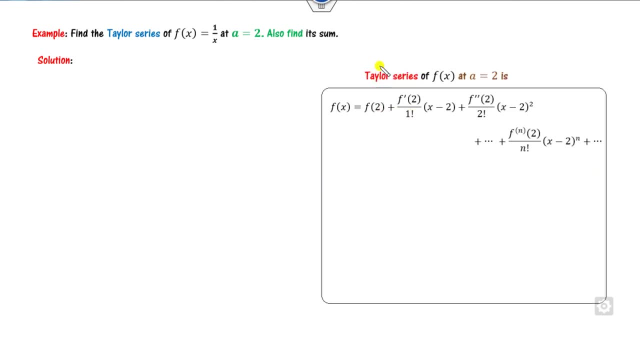 n and so on. So it means your target is to write the Taylor series above the 2 here. So what you can do, you have to find the derivatives of x, 1 by x whole. So this fx. this is the first derivative. this is the second derivative. 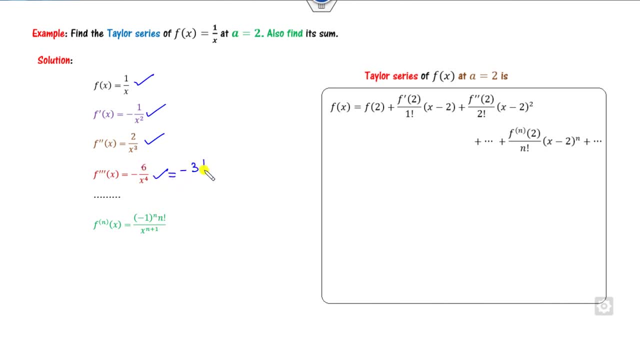 And so clearly say that I can write 6 as my 3 factorial over x, 4.. This is my 2 factorial over x cube. This is my minus 1 factorial over x square, and so on. So you can say it's a plus, minus, plus. 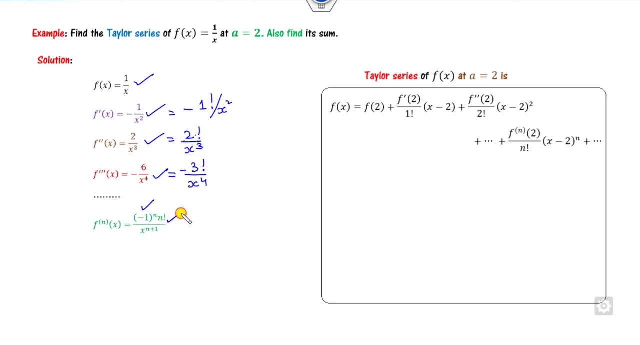 minus. So it is here 1 factorial, 2, 3 and so on. So if it is a 3, then it's a 3 factorial, it's a 2, it's a 2 factorial, but the denominator power is 1 addition of this one, So n plus 1.. Now we can. 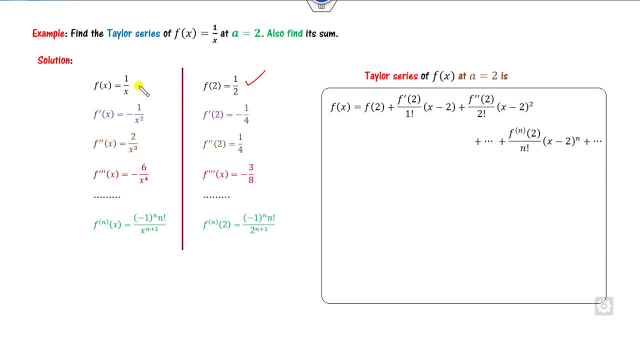 compute these factorials, So we can write these values at 2.. So what is the f of 2?? You can substitute here. You can find all these values at here. Substitute this value. in this case you will get this expression, or this is a: 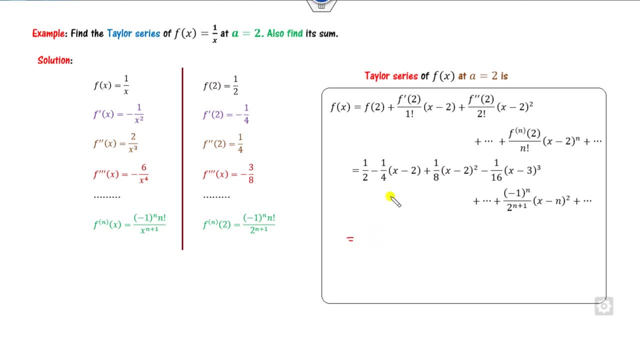 power series. this is a Taylor series of this one or otherwise. you can express more. You can see, I can write this 2 as here. I can write this 2 as 4.. I can this as cube. I can write 8.. So I can take. 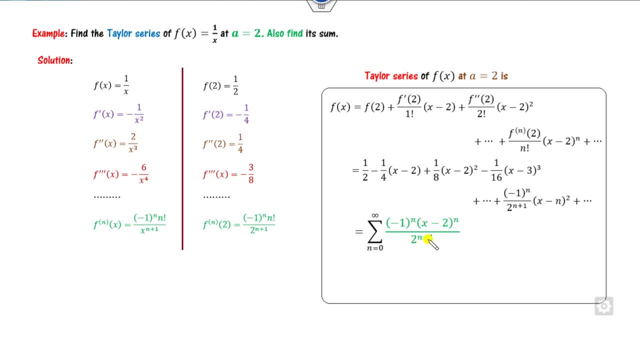 1 by 2 as a common, or you can write this series as Here. Now, another target is how you can find the sum of the series. So do you think that, whether this is my arithmetic progression is a geometric progression, and so on, How you can find that? 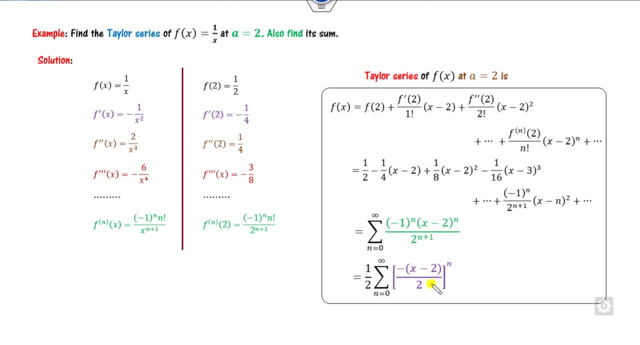 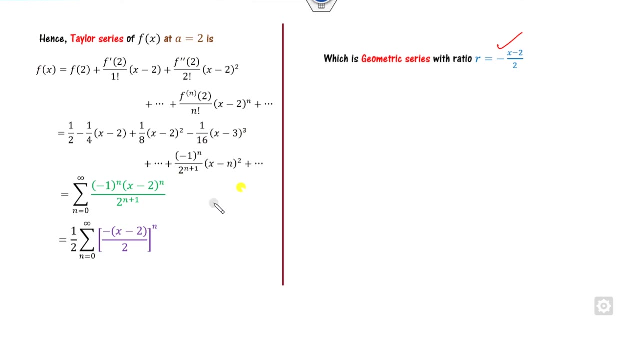 clearly say that this is my. here. you can write this bit by: So what is that? this is nothing but my gp series. So once you know that it's a gp series, how you can find the sum of the infinite? So this is a over 1 minus r. So that is, r is my common ratio. 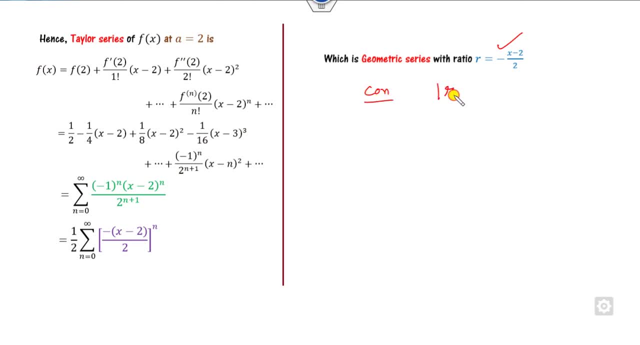 And when it will be convergent. We all know that gp series is convergent when mod of r is less than 1.. I can substitute this value here. We will get the. this is the value of the x for which series converges, And the sum will be a over 1 minus r, So half will be outside. So this is the. 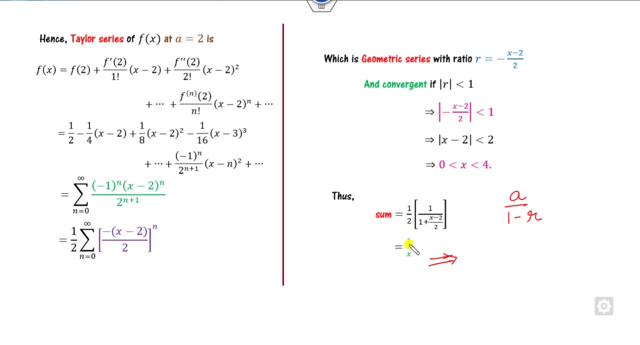 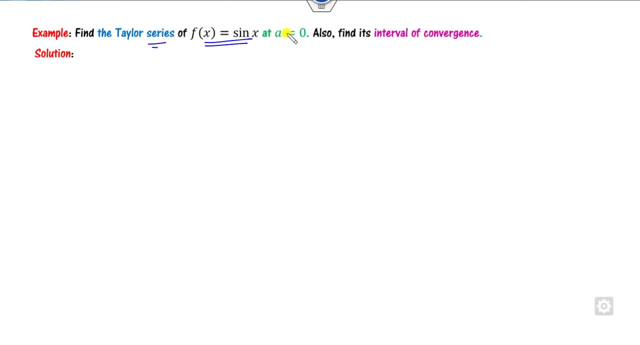 right answer of this And you can see the function value is: sum is 1 by x. Look at another one Again. this is a over 1 minus r, So half will be outside. So this is the non-polynomial. So you have to express the Taylor series Now. this case is: a is equal to 0.. 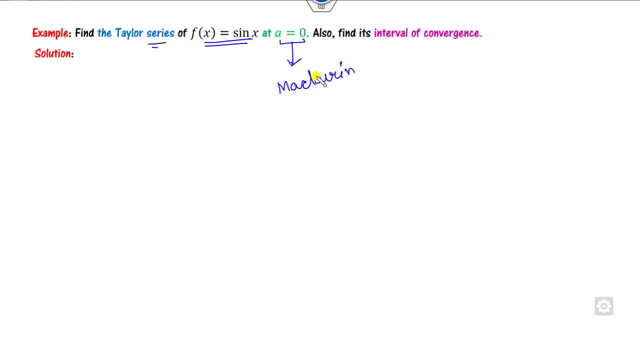 So basically, your target is to find the Maclaurian series of this fx. So this is the target, because at the point f0. So we can find the derivatives, all those derivatives of fx, f, dash, f, double dash, f, triple dash, and so on, You can find all those values at the point 0. So sine 0 is 0. Cos 0 is 1.. 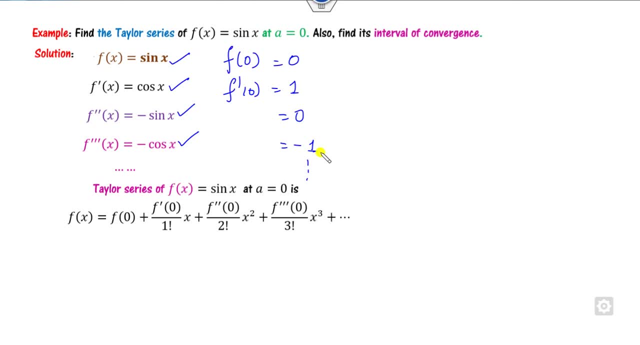 Sine 0 is 0.. Cos 0 is minus 1.. And so on. Substitute value here f dash is 0. This will be 0.. This will be 0. And so on. You will get this series. So that is what is. fx is sine of x. So that is my Taylor series of sine x. 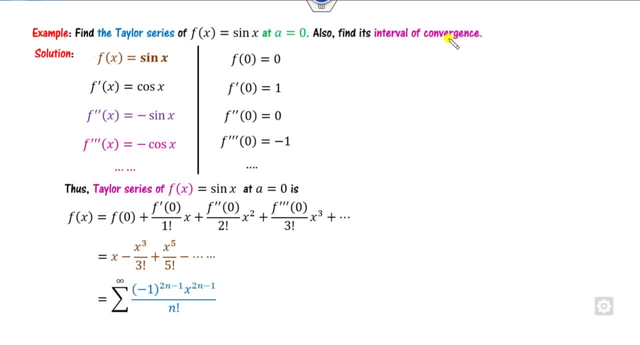 Also find the interval of convergence. So how you can find the interval of convergence In journal, you can write like this way: How you can find the interval of convergence- That we already discussed in the power series lecture. We can start from here And if it is less than 1,. 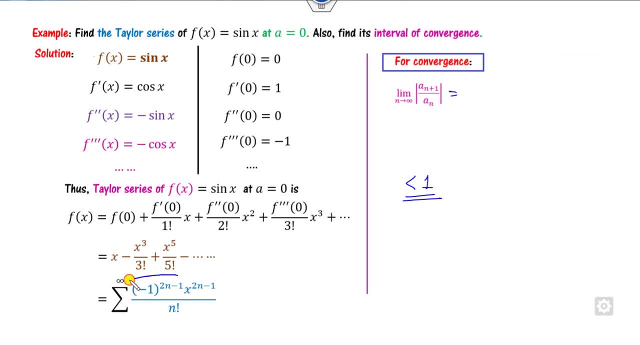 we can find the interval of convergence. So what is the a? is This is my a- n. So what is the a? n plus 1? You can substitute this value here, So you clearly say that this will be cancelled out. It come out to be n plus 1. only This will be cancelled out. It give you x square Because of. 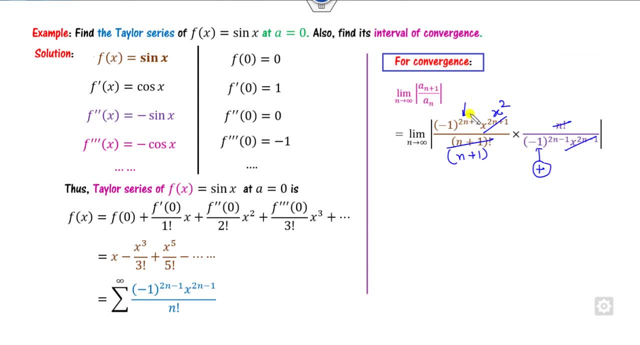 this modular sign. this value is my positive, This value is also positive. So what is the answer? is my here? Take n approaches infinity. This goes to my 0. And 0 is my less than 1.. So what is the meaning of the less than 1?? That means by using the ratio. 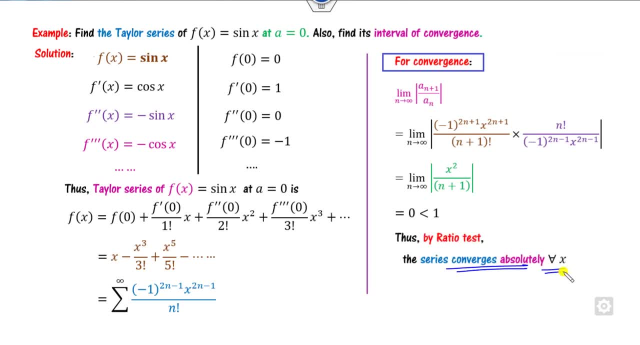 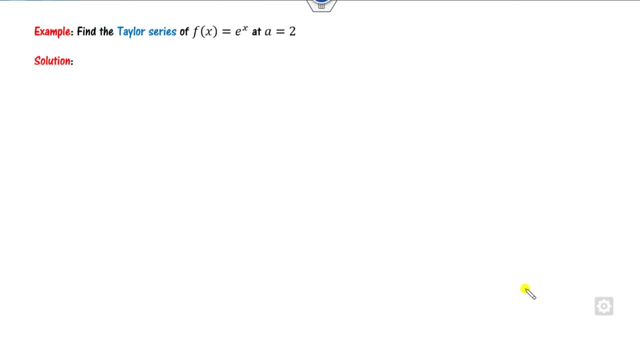 test. this series is convergent for all value of the x. That means sine x is convergent for all the values of the x. Look what is another one. That is a Taylor series: e raised to power x. Now you have to find the value at a is equal to 2.. So you can find the first derivative. all You can find all. 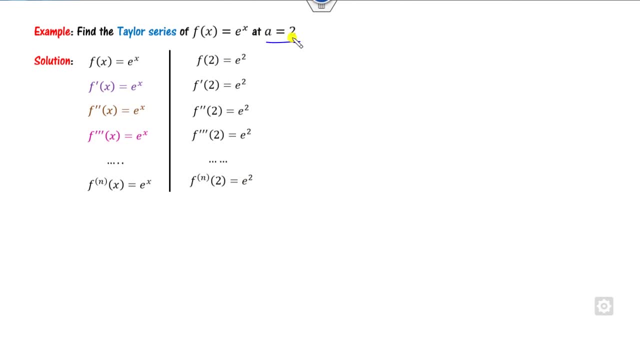 these values at the point 2.. You will get same Now the Taylor series about the 2.. That is my here. You can substitute: This is my e square. This is what is that. f dash is e square over 1 x minus 2, and so on. You can take. 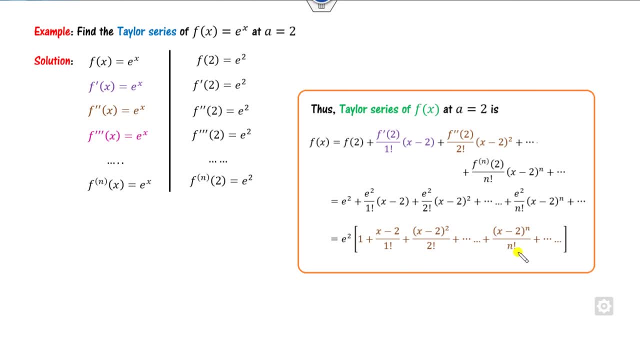 e square as a common, You will get. this is the series, Or you can write this number, as this is series of x minus 2 raised to power n over n- factorial. So you can take n is the first number is 1.. So I can take this number as a. 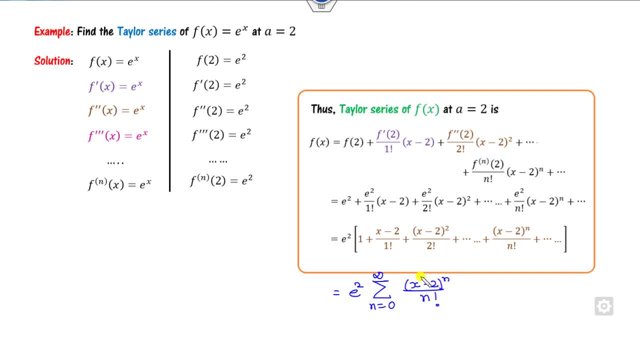 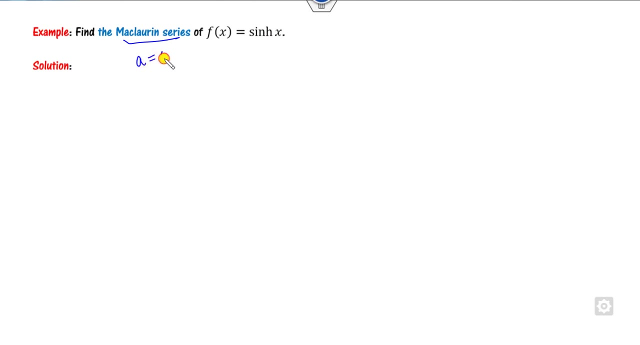 0 to infinity. So this is the required series of. here You can also find the interval of convergence. You can take this value as discussed in the previous one. More of this are here. Look at the Maclaurin series. That is a Maclaurin series. That means you have to find the center at. 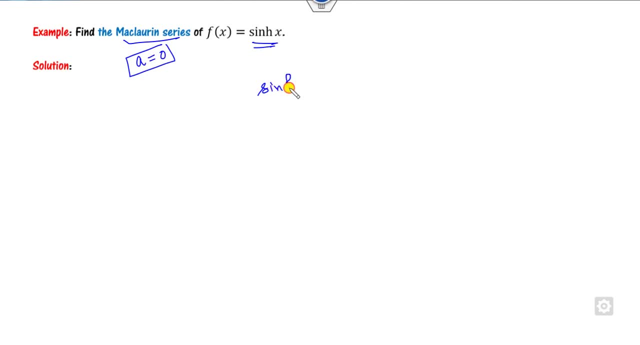 0. What is the sine h, Sine hyperbolic x? So we all knows. I can express this in terms of the exponential. This is my here, So we can write Maclaurin series. Take f of x, is this? Find the derivative f dash, f, double dash, f, triple dash, and so on. You will. 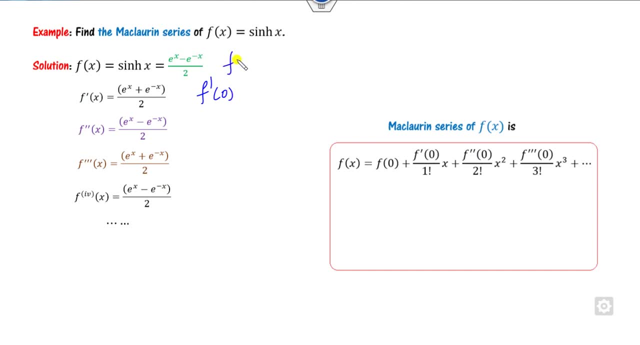 get here, Find these values at the point 0, at the point 0, and so on. You will get: this is 1 minus 1, 0, and so on. Substitute this value here. This is my 0.. This is my 1 over 1 factorial x. This is: 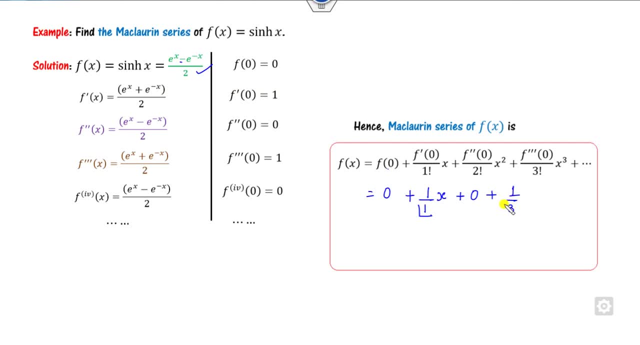 0.. This is my plus 1 over 3 factorial. x, q. you will get this as the series which can be summarized them here, because this is the odd power. I can write this as 1 factorial and so on. You can find the Maclaurin series of the cos square. 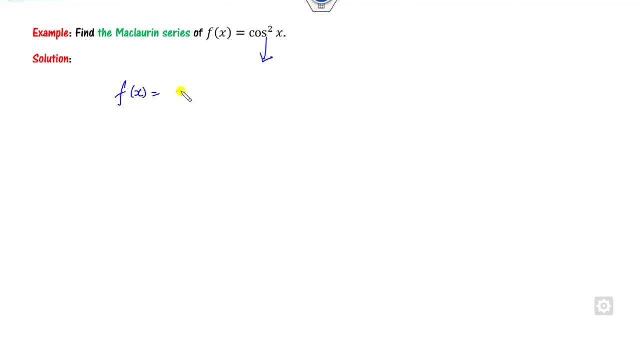 so how you can write this as a cos square. the first method is you can take f of x as a cos square. then you can take that second derivative. first derivative is 2 cos x, minus of the sin x. then second derivative: or you can write this as minus of sin 2x, then it's minus of 2 cos x. 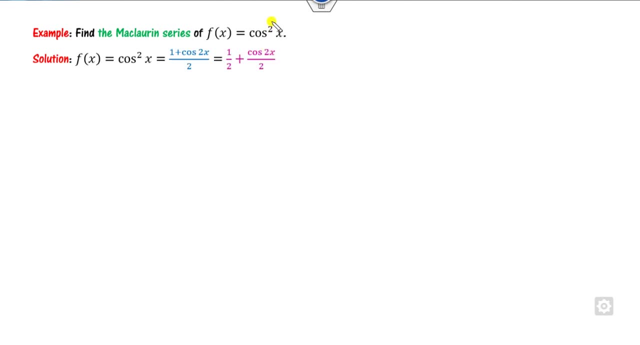 and so on. Otherwise we can open them as a cos. square is my here, since this is my constant, so I can write this as a polynomial: series x raised to power 0. this is already in the form of the x we can find only for the cos here, cos of the 2x as here, So I can consider this function as fx. 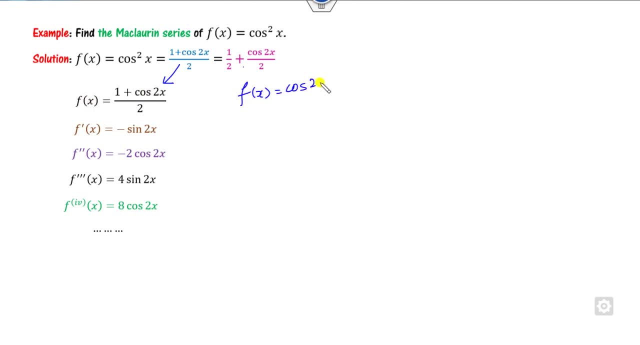 or you can simply consider this as a cos of 2x. We can take the derivatives and then we can find the values. at Maclaurin it's a 0. we can substitute this value of this. So f of x is my here. you can substitute this value. 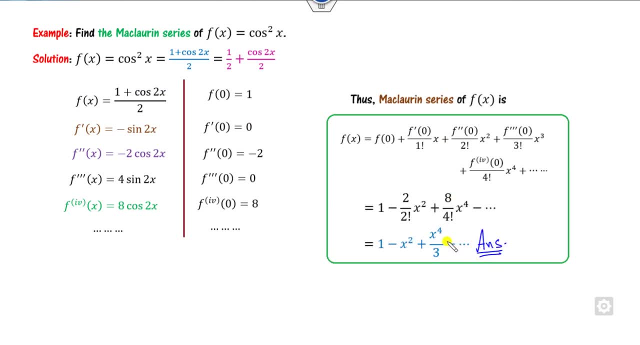 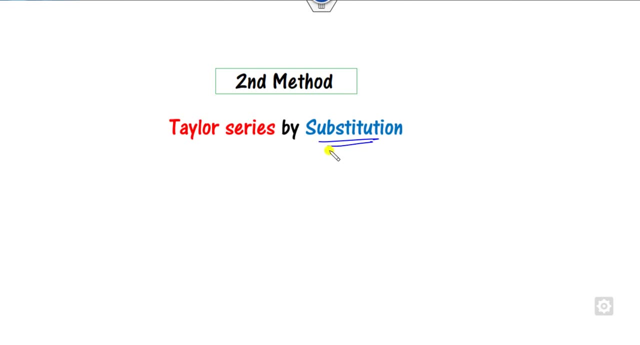 you will get the required answer of this series. Now this is another method of the Taylor series. you can use them, the substitution method. that is quite easier to solve them. How Look at it? Now? you can see this is the product tool piece, The first method. 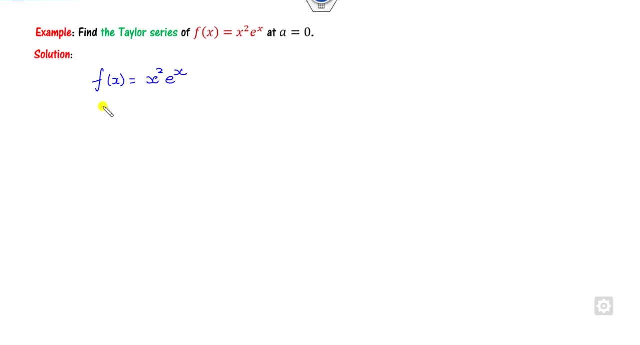 as a cos of 2x. We can take the derivatives and then we can find the values at Maclaurin, as we discussed in the previous case. that is, if you take this one, you can take the first derivative, that is, a 2x e raised to power x plus x square e raised to power x. then second derivative in the 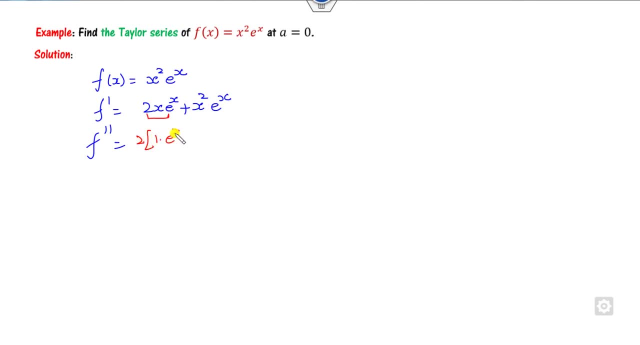 second derivative, again you have to take 1 into ex plus x into ex and again here as a product rule, and it will take a lot, of, lot of calculations. so, apart from them, what you can do, you just think about here term, so you can see this is already a polynomial, so there is no need to find the 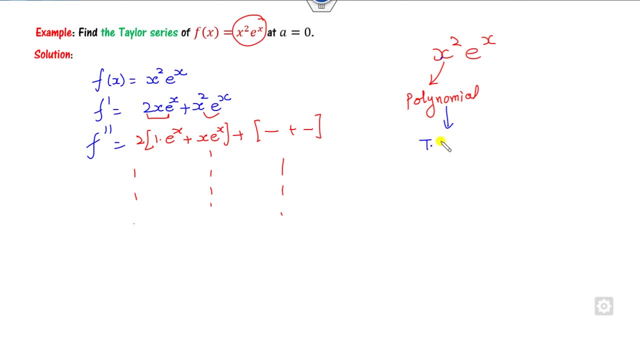 taylor series corresponding to this, because the taylor series corresponding to x square is itself x square. it is already a polynomial about the 0, so this is a non-polynomial. so we can firstly find the taylor series of only gx. so what we can do, we can take the gx is e raised to power x. 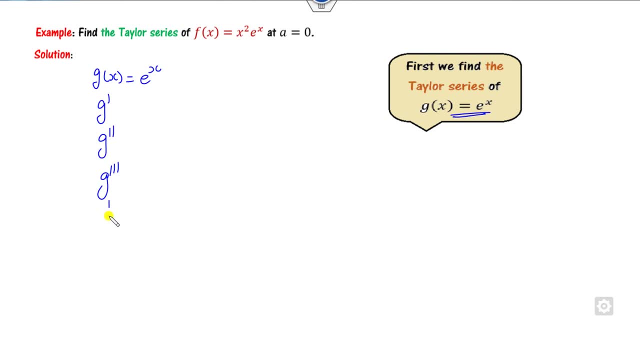 we can take the first derivative, second derivative, third derivative, and so so, since it is the same. so we have to find the taylor series about 0, we can find the g0, we can find the g dash, 0 and here. so, therefore, the taylor series about the. 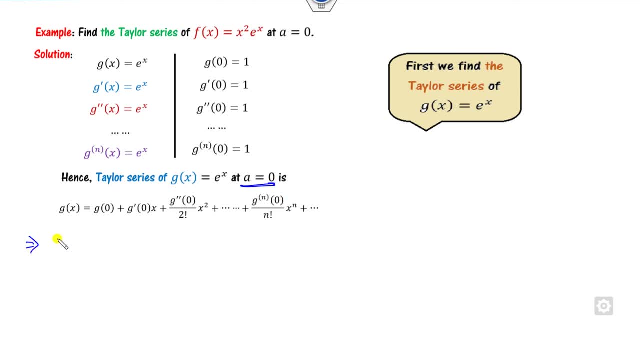 0 is my here. what is the gx is gx is my e raised to power x. g of 0 is my 1, this is x, this is x, square over 2, factorial, and so on, or in general. we can write this number as here. so this is the mclaurin's or taylor series of the e raised to power x. now we can multiply this by: 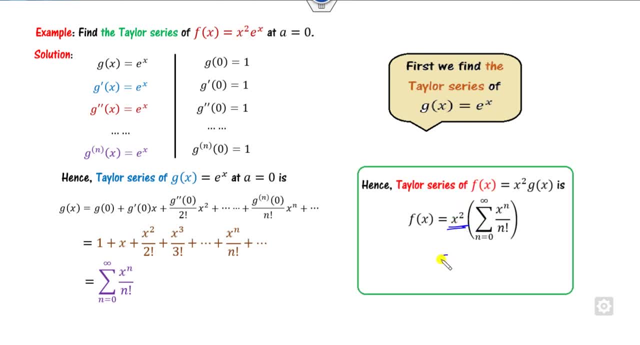 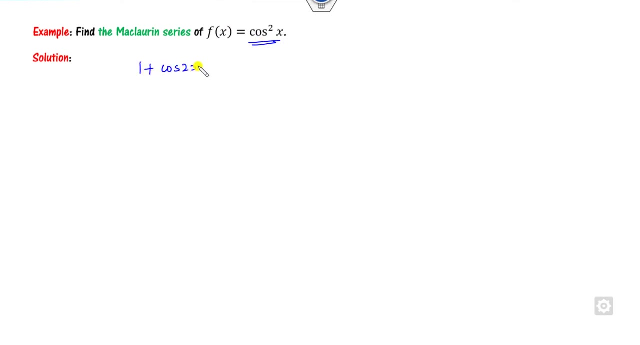 x square, because this is already a polynomial, so we can multiply them. what will happen? this is my required taylor series of this polynomial, of this function. look at this function. the first method we already discussed in the previous question: we can solve this question like of this, we can take them and so on. but the another method is: we can because this: 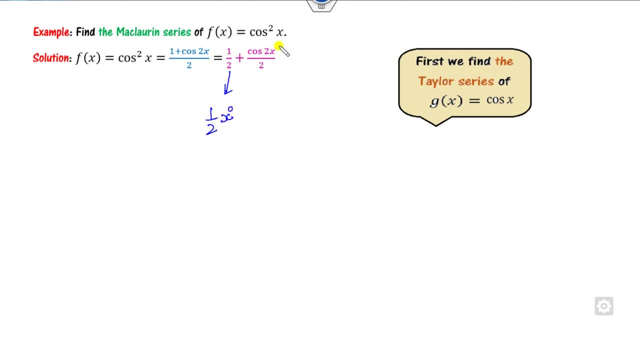 is all a constant, which is a taylor series already. another method is: we can try to find the taylor series of cos x. only how you can find the cos x, although it's a 2x, but we can find the cos x. so this is the derivatives we can take here and we can substitute this value in the taylor series. 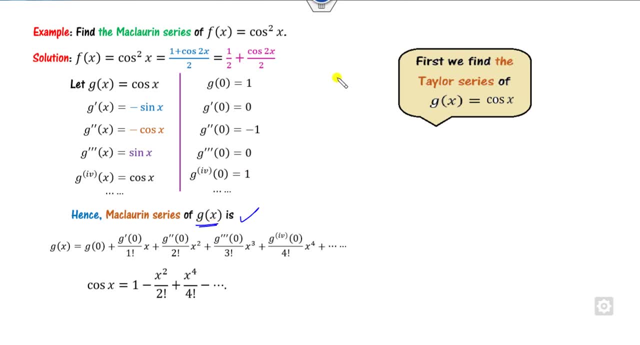 so this is the mclaurin series of g. that is a cos x, but we need the value of 2x. so what is the mclaurin series of the 2x? i can replace x to be a 2x. so once you know, the cos x, cos of 2x is there and this is on itself a taylor series. 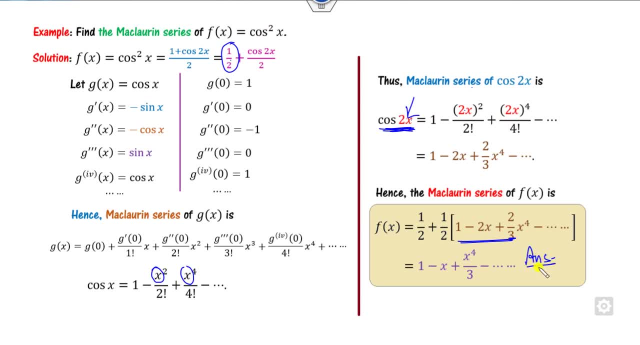 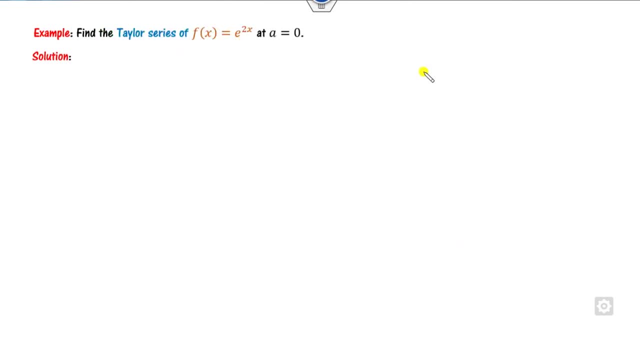 i can substitute this value and you can see both. the answers are same as discussed in the previous. again, e raised to power 2x are there. so the first method is you can take f of x. is my e raised to power 2x? then take the first derivative here. second derivative: